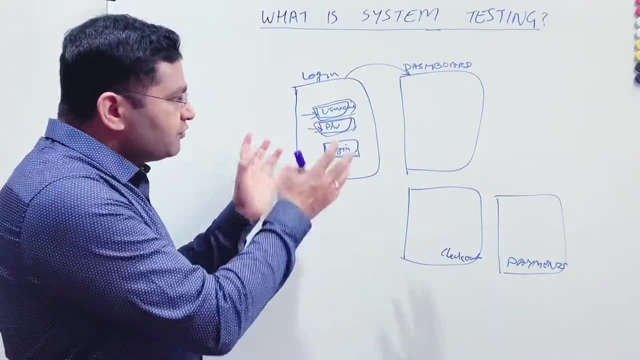 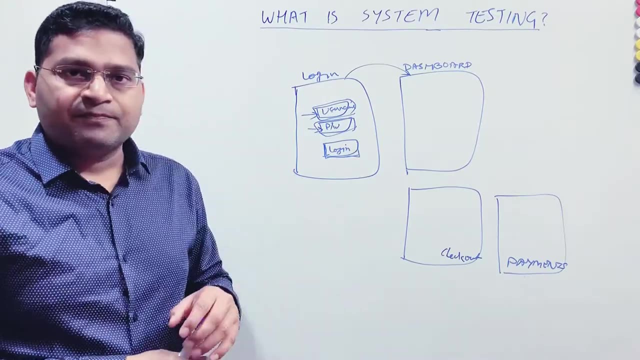 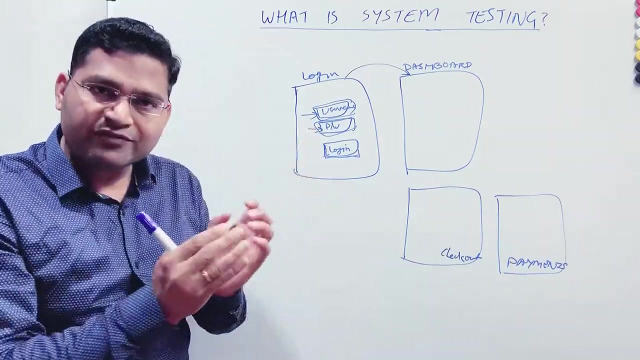 what integration testing is right. So a couple of units integrate together and you're testing those couple of integrated units. Now, when it comes to system testing, system testing is testing system as a whole right Now. in this case, if I'm just testing login functionality of the overall 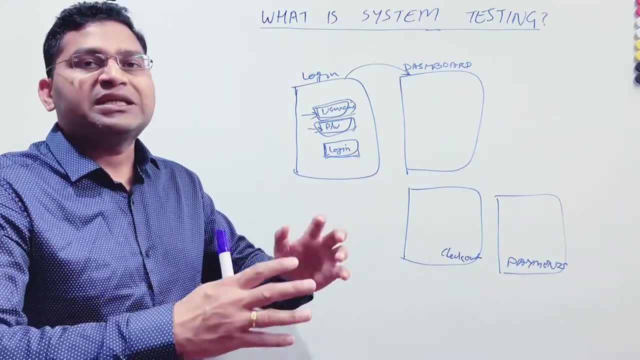 e-commerce system, then I'm just testing the login functionality of the overall e-commerce system. If I'm just testing the login functionality of the overall e-commerce website, that is not the complete system. right, Complete system is the complete e-commerce website with all the functionalities. 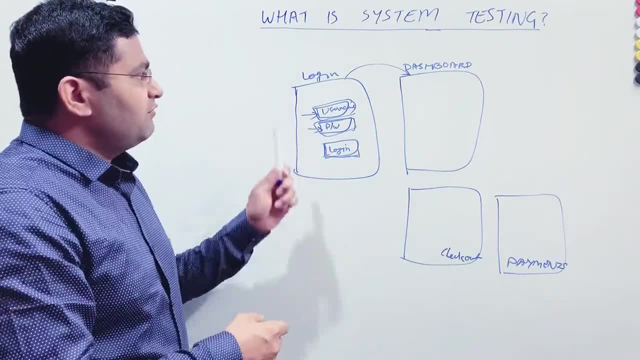 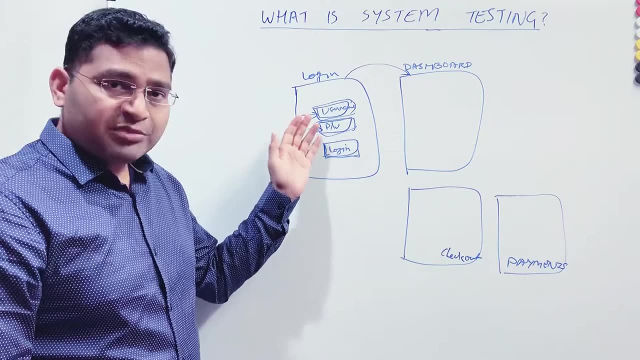 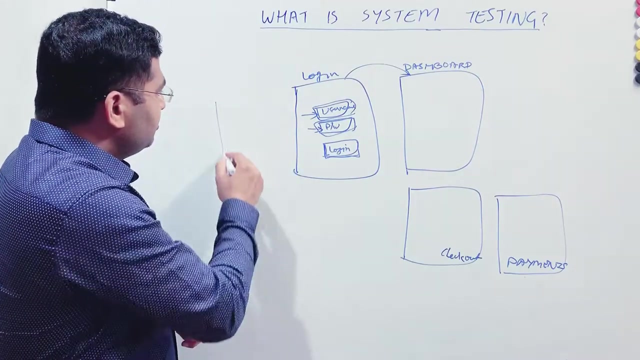 that have been requested. So a e-commerce website can have login functionality and login even in the login functionality, I can log in or register using email or I can log in using my social media account, right? So login functionality is one. Then, prior to that, there is a registration. 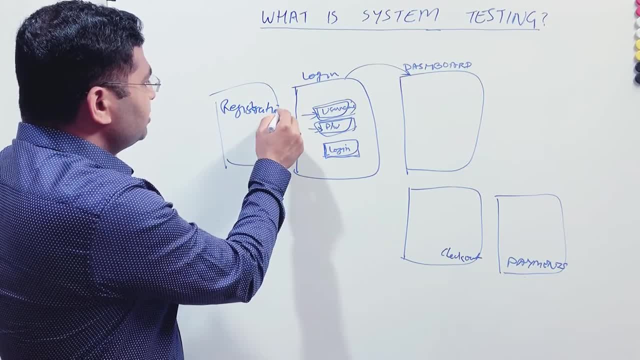 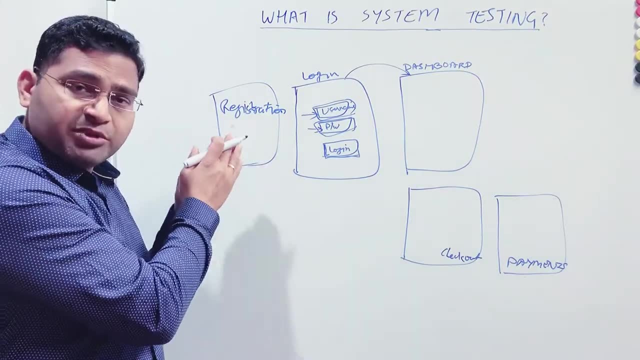 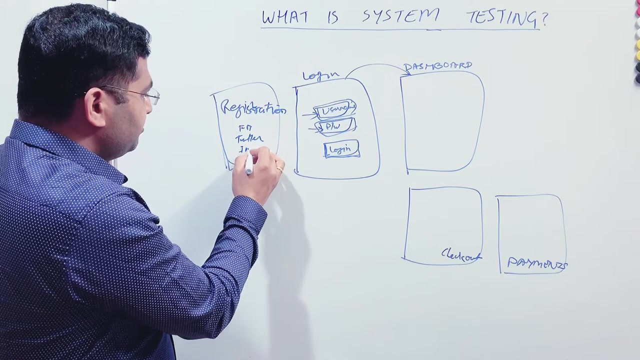 functionality as well, right. So registration, when we, when we say register user, so the user can register using email, his email, or through the social media accounts, for example, FB, Twitter or Instagram. okay, So Google, so all these are social media. 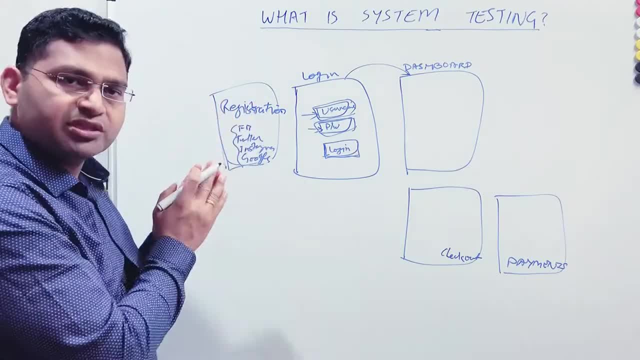 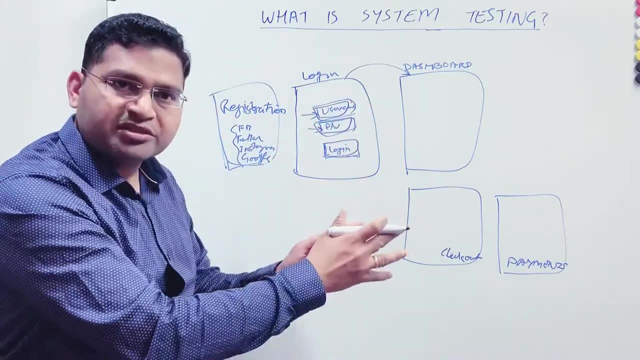 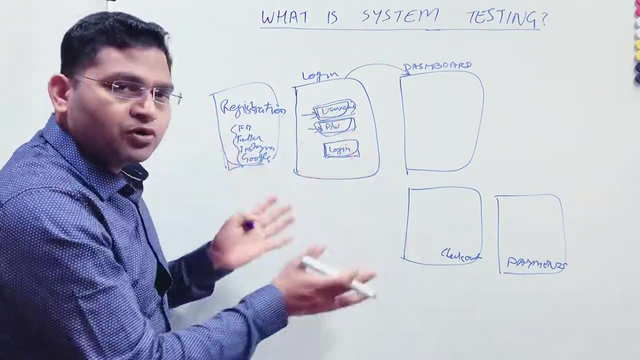 login possibilities or integration possible on the registration page. So this is one of the modules, the login is another module. dashboard another module: checkout. payments, add cart, remove cart. there are so many modules or features that will be there in the overall e-commerce application or system right Once all these modules are integrated. 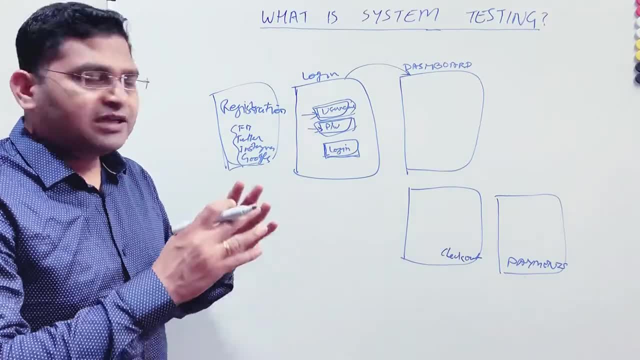 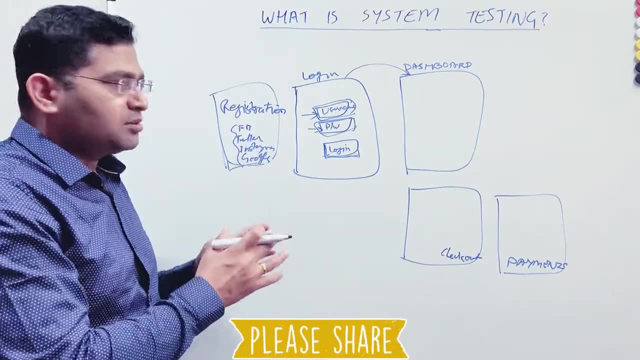 together and working fine, and you are testing that. this is. you know, the integrated system as a whole is known as system integration, So the integrated system as a whole is known as system testing. right, So, taking back to the car example, I have tested the wheel, so which is? 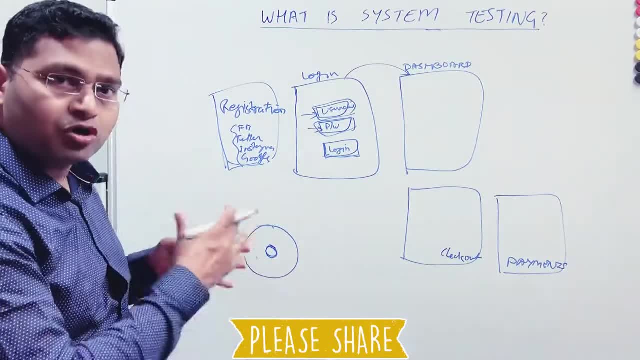 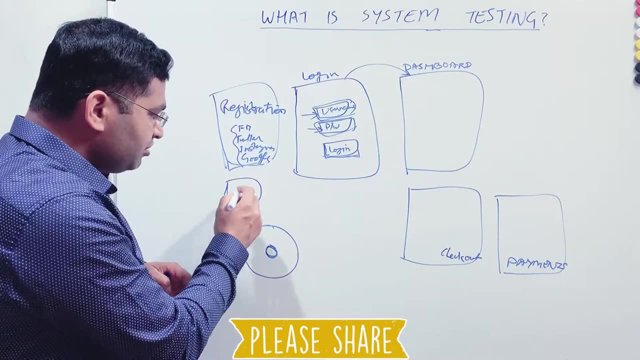 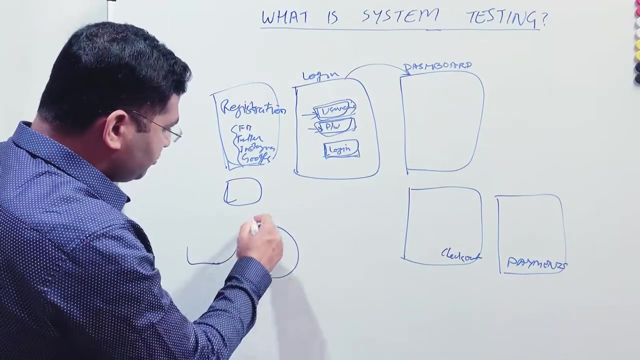 integrated system, all right, Or integrated, you know, or integration testing, basically of the wheels. When I have tested the wheel, then I'll test the integrated engine, right Then for the body, there'll be, you know, like testing Once all this is assembled together, okay, in the car. 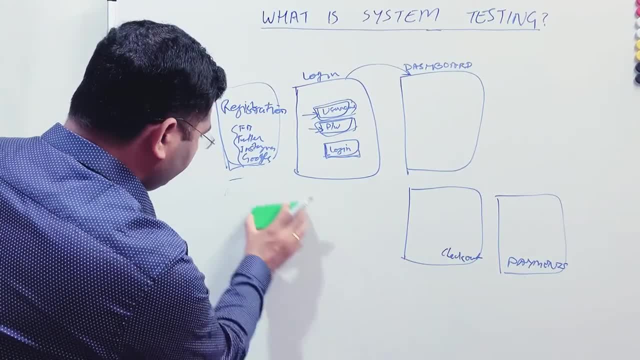 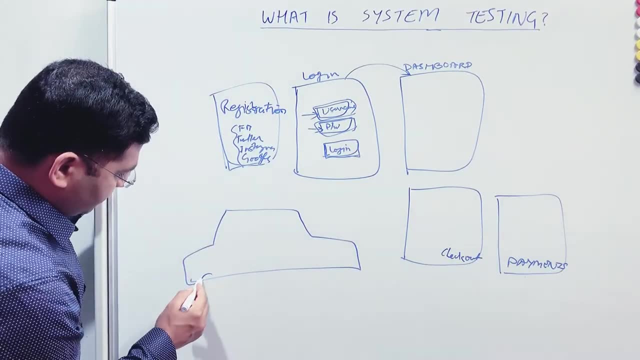 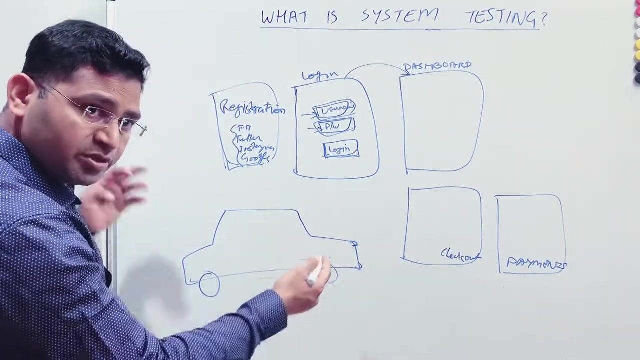 let me make it a bit small. So say, for example, this is my car, So this is my car body. Then the wheels are fitted here. You know all the headlights. these are, you know, like small units, and there could be even. 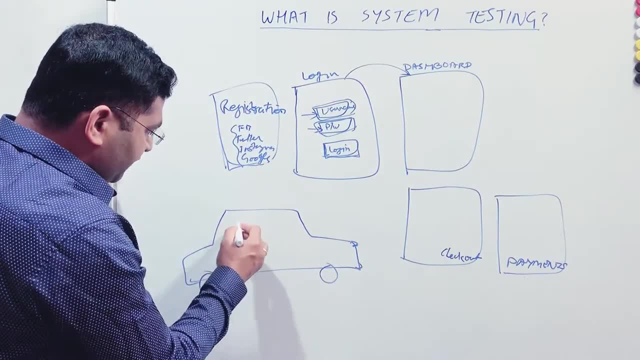 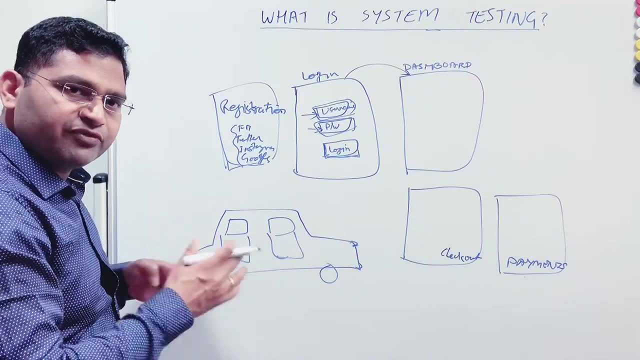 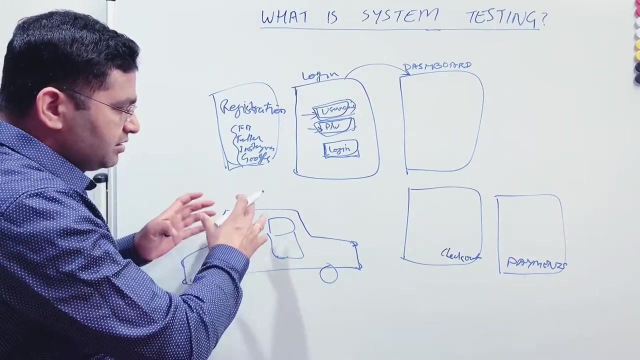 more small units within these small units: The window, the door, everything once has been built and tested how everything is, you know, integrated and available within the car, Once the car is is ready and needs to be tested as a whole. this is what the system testing will do all about in. 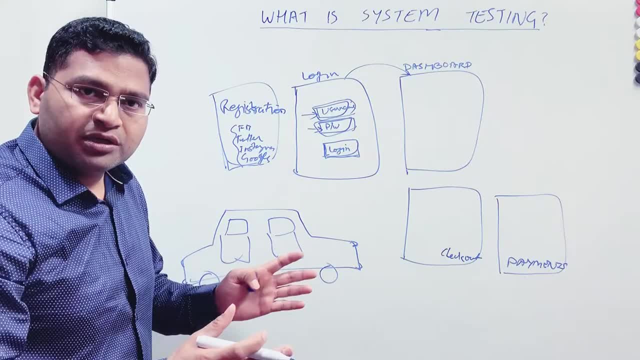 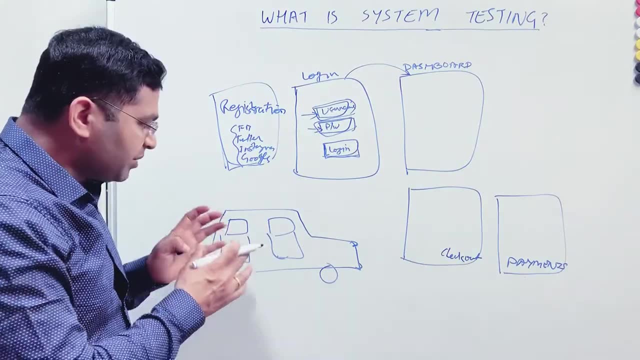 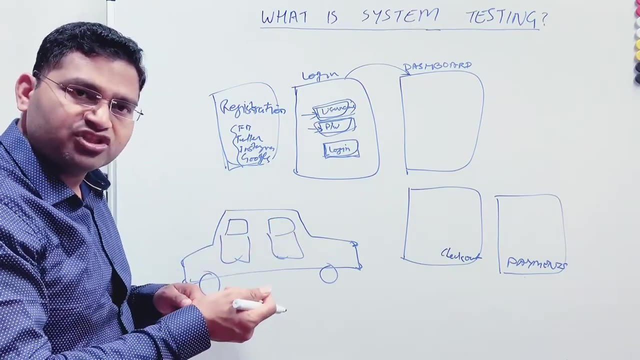 terms of car right. so when car is ready as a whole, it's moving and all the you know functionalities are being implemented, all the parts are being put in place in the car, and then i'm trying to, you know, test the car, i'm trying to turn on the engine and then accelerate, i'm trying to, you know, ride. 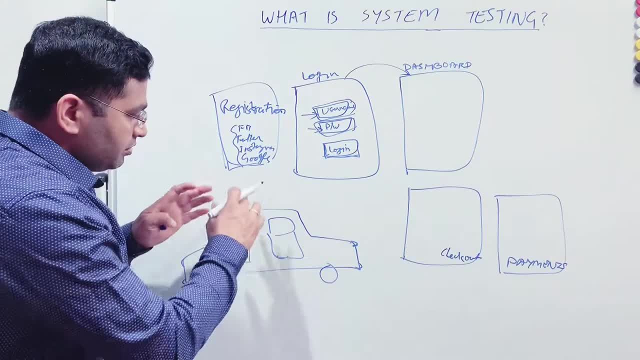 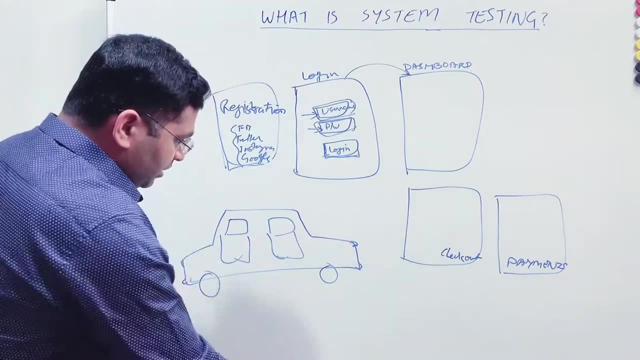 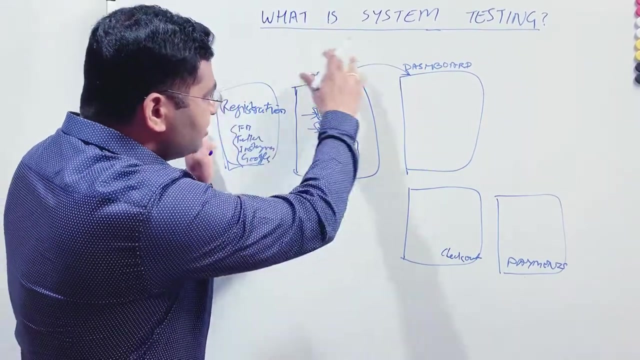 the car and see how the performance. i'm trying to break it- that whole testing, or testing the car as a whole, is system testing. all right now, taking this same example back to the e-commerce website, when we integrate all the functionalities that need to be built on the e-commerce website, that 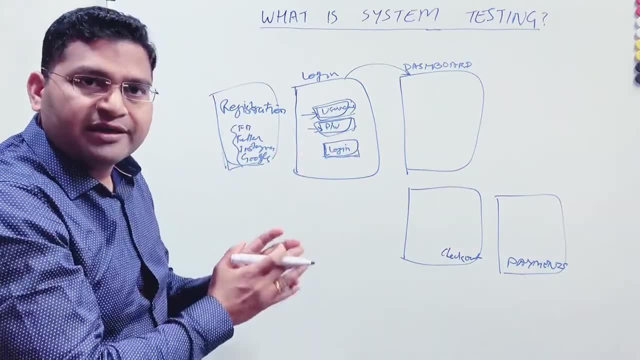 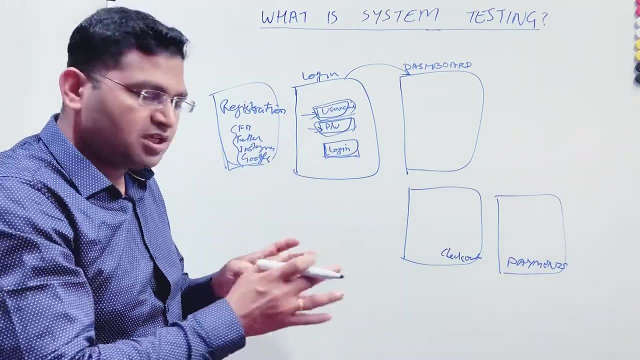 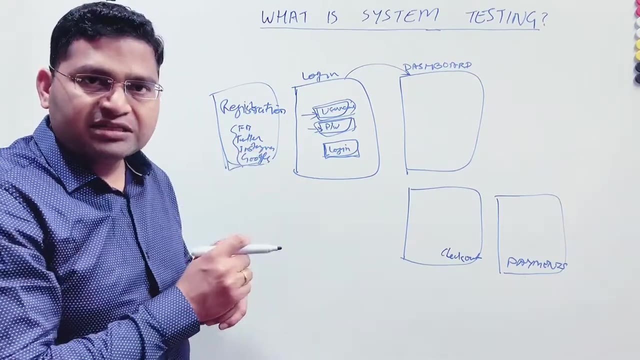 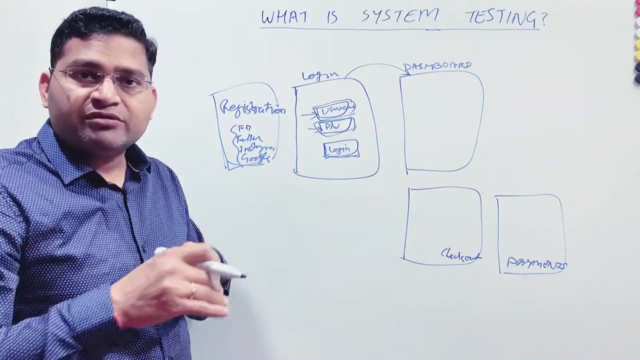 are given by the customer. all of them are integrated, and i'm testing that integrated e-commerce website on the test environment that has been deployed there and i'm able to do end-to-end test cases there with all the functionalities there. then that is what system testing is all about. now, system testing can have system testing and system integration testing. 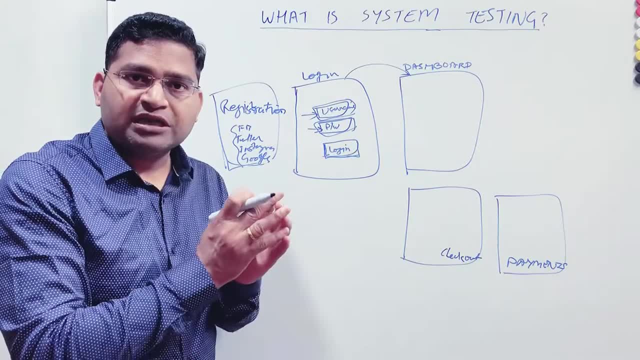 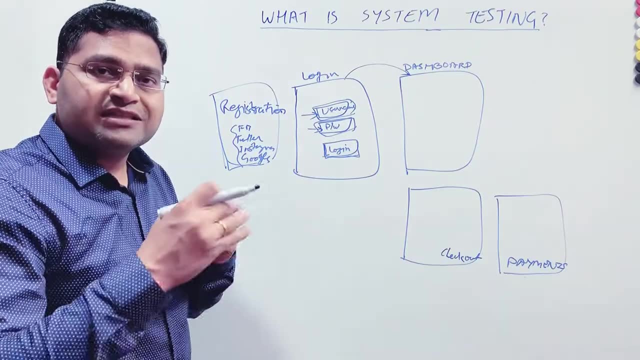 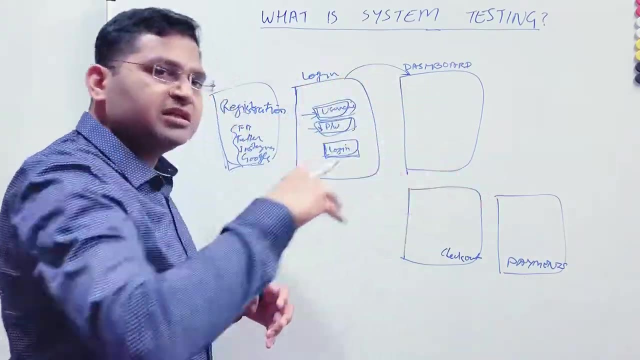 sit as well. if say, for example, your e-commerce application integrates with third-party systems or external systems, then you have to do system integration testing as well, because in that case your system, e-commerce website, need to integrate with third-party system or external systems as well, so that part needs to be covered in the system.